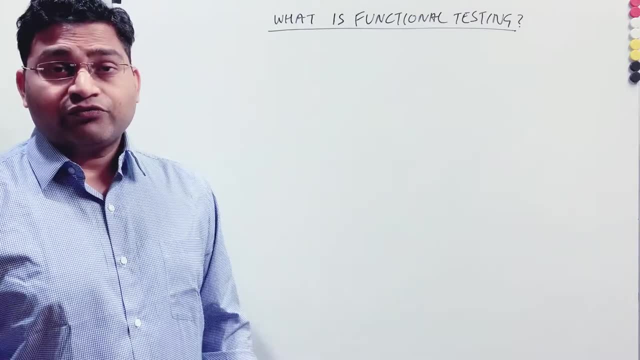 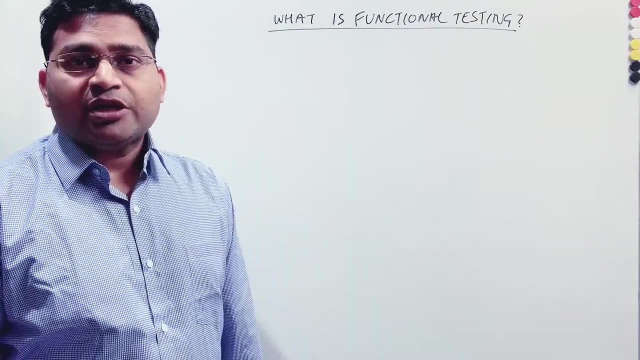 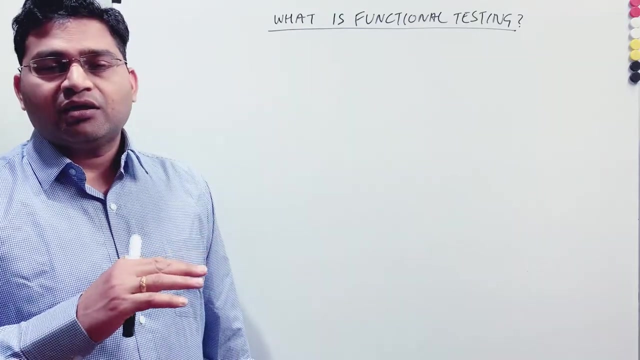 Hello everyone, welcome again. In this software testing tutorial we are going to learn what is functional testing Now, in the previous tutorial I have explained about the types of testing already and I have briefly covered the functional testing as well and briefly also explained about. 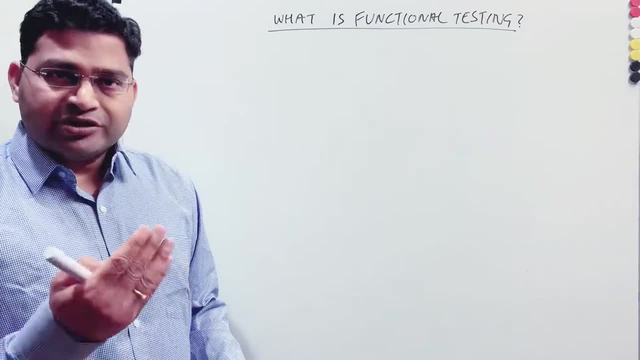 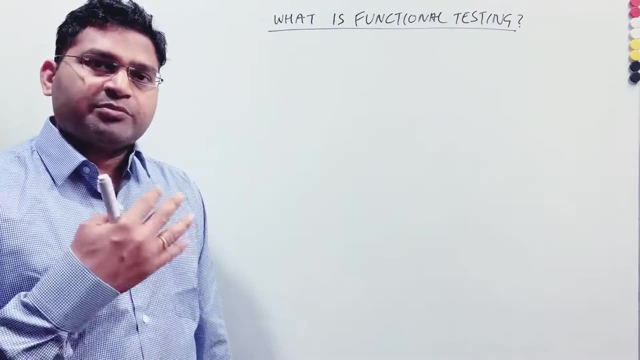 the difference between the functional and non-functional testing. Now, in this tutorial, what I'll cover is I'll take the real example and I'll show you what exactly functional testing means, along with the definition of functional testing. Now, if you see the functional testing, 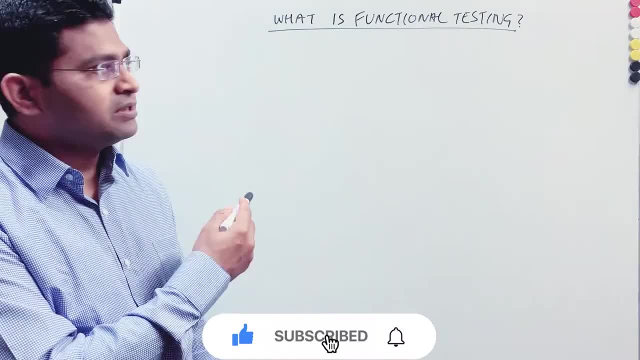 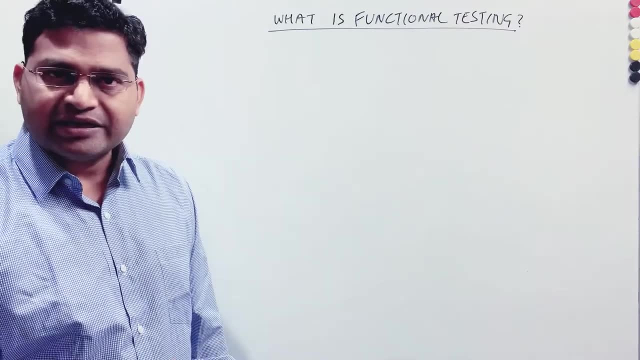 word itself defines the functional within it right. So when we say functional testing, it's basically testing the functionality of the application. Now, if you take any example of an application, say, for example, I'll take an example of the Gmail in this particular tutorial. Now, when 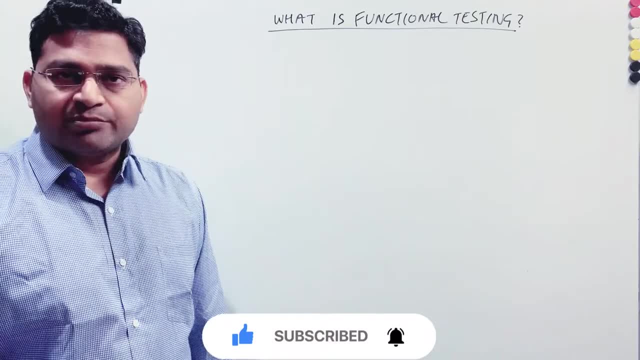 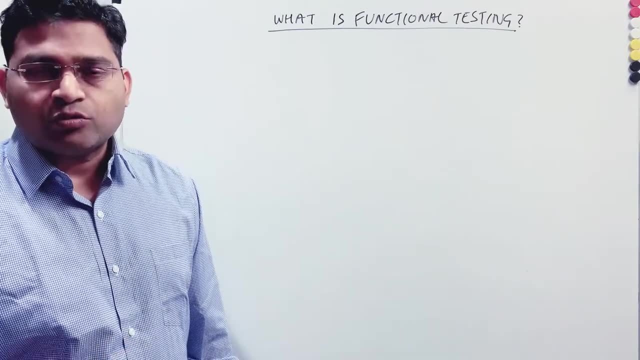 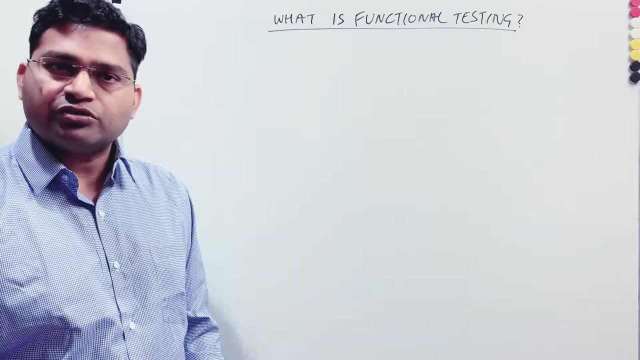 we launch a website or gmailcom in any browser. if you don't have an account, you click on create account. Then it redirects you to the create account page wherein you can provide all the username, password, all details and click on create account and it creates account for you, right? So this? 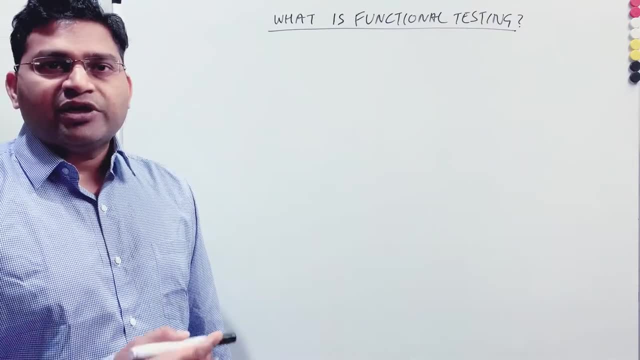 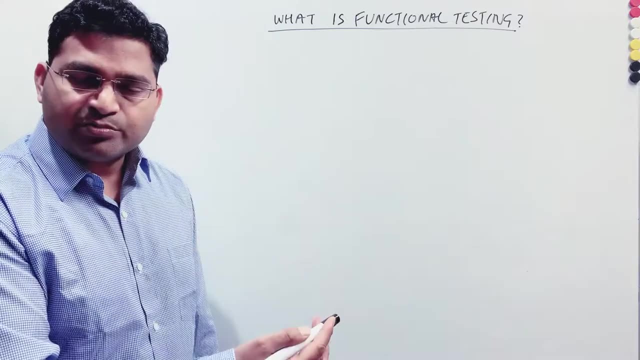 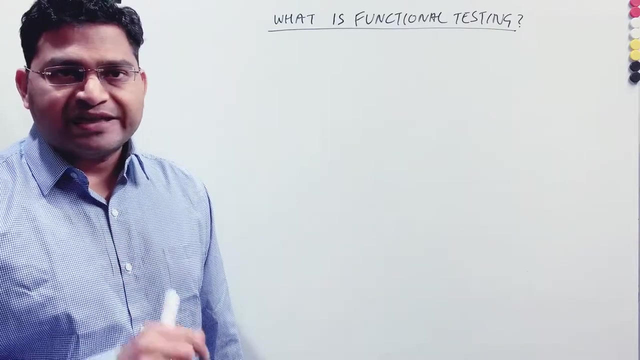 whole process that you follow is basically verifying or, you know, creating the account or this type of testing that you do in the any test project. is the functional testing right? In this case, you are not worried about one once you click on create account. how much time? 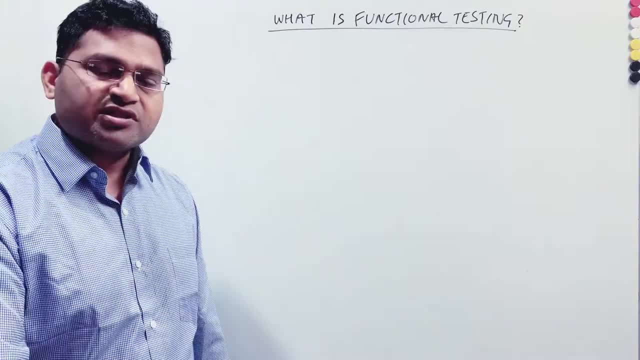 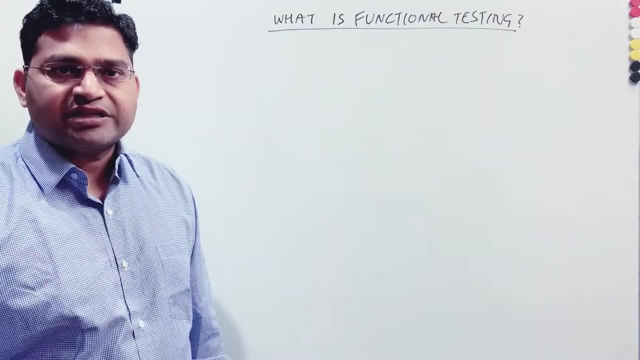 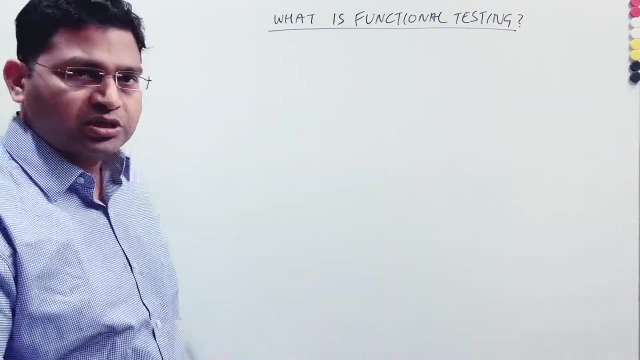 it takes to actually create the account. That's the non-functional aspect of the create account functionality, right? So when we say functional testing, it is verifying the functionality of an application. Now how will our how these functionalities are being built Now? usually, 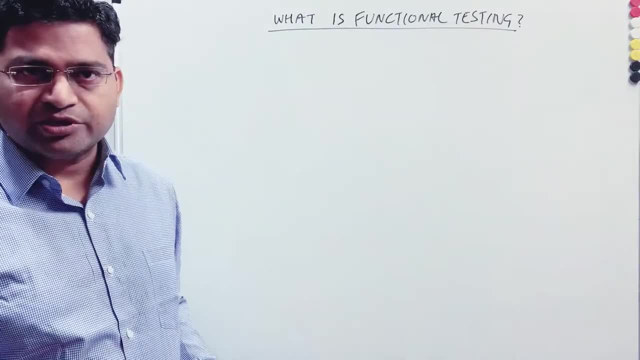 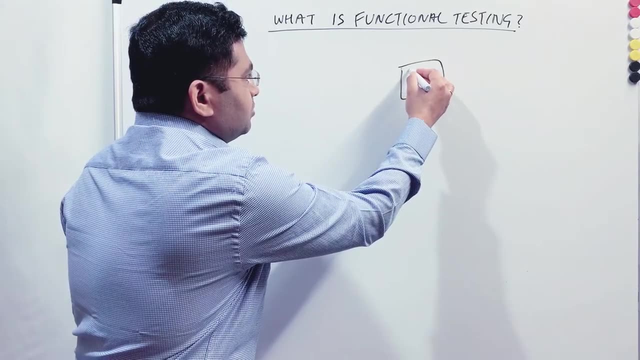 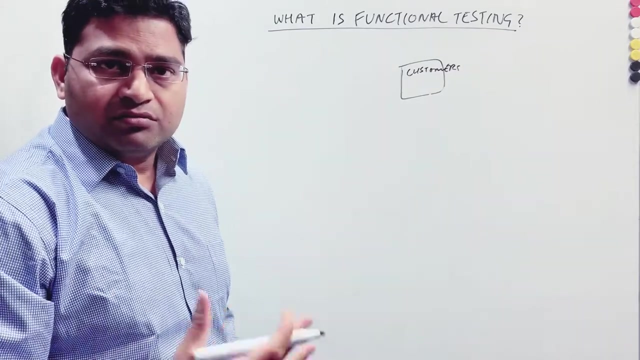 in case of Gmail say, for example, we are the customers, right, The end users are the customers, So we'll be having you know, customers, So customers right. And if Google is building the Gmail or email client for the customers? 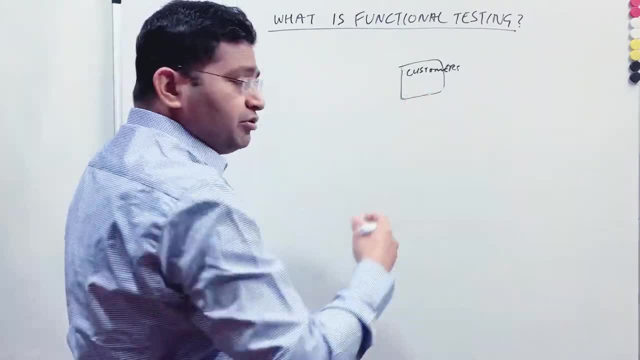 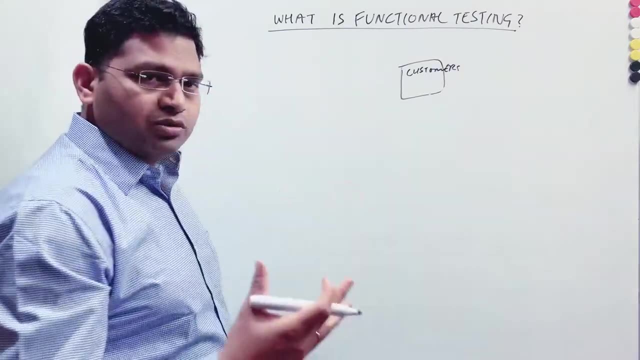 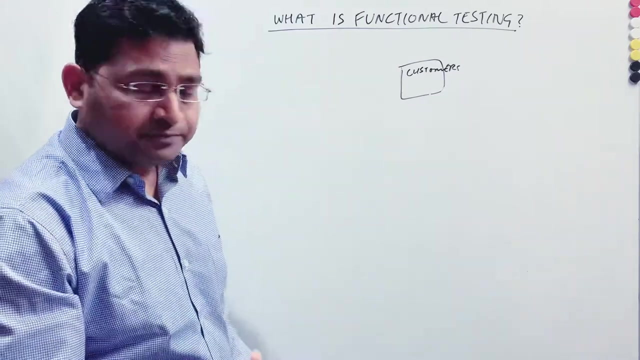 which is basically the general public. then they will do a basic research: what all things are missing in the application right. So usually in the actual you know projects or many projects that you would be working in, customers might be either the general public, for example, in case. 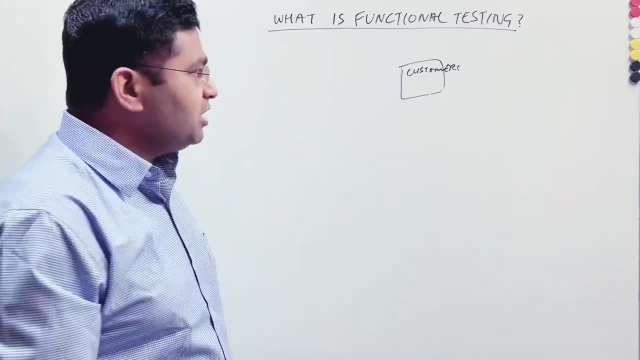 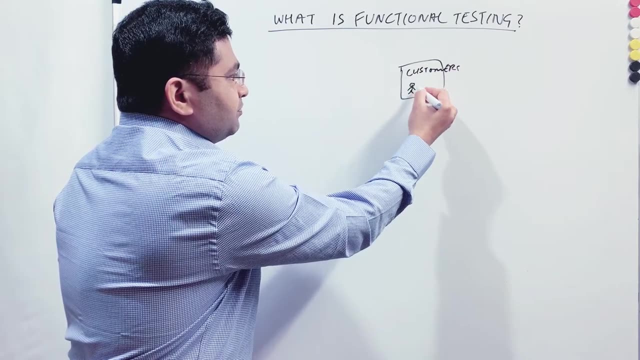 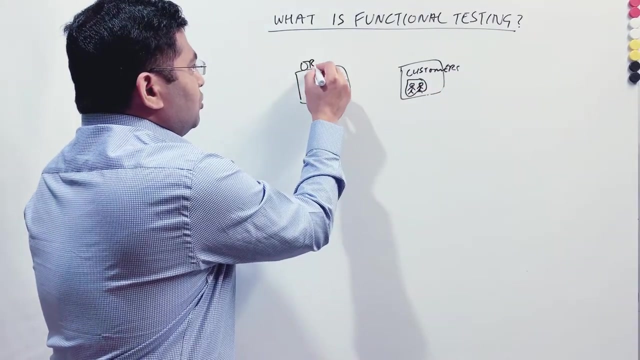 of Gmail. people like us Who will be using Gmail or customer, can be a company, And within a company, there could be, you know, like people and the team who will be providing the detailed requirements to the organization who is building any software right. So we are the customer. Let's take an example of 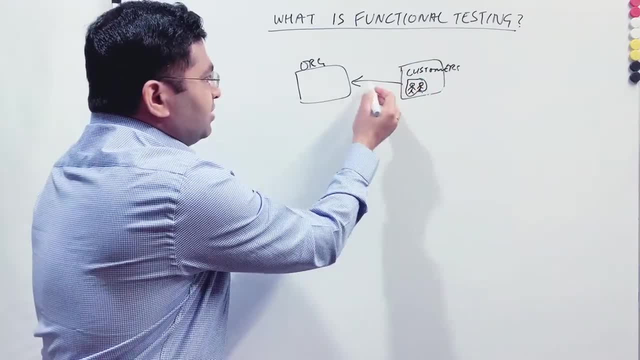 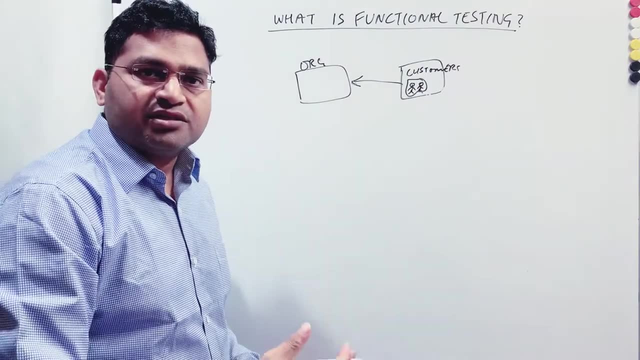 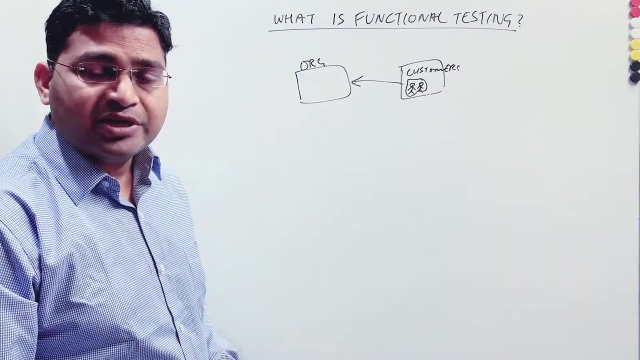 the Gmail. We are the customers, the end users, And what Google has done- they had done the market research. They have researched the existing softwares that are available or the email clients that were available at that particular time, what all limitations were there And, based on that, 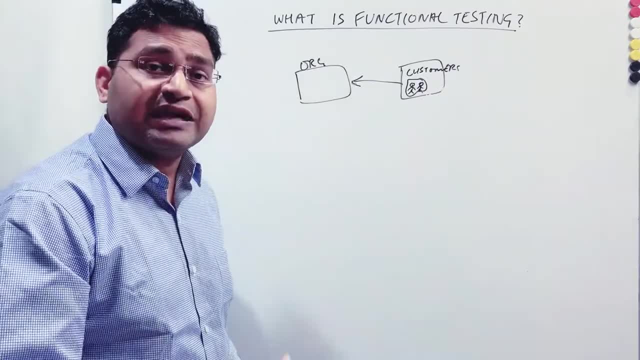 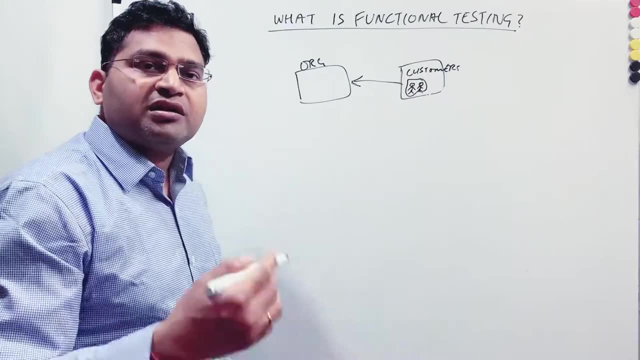 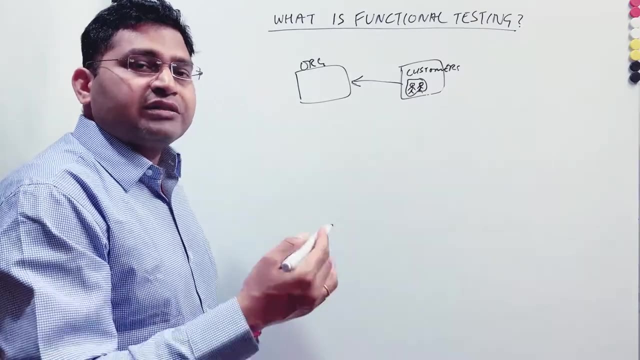 they came up with the functionalities that they need to build in that particular application right. So usually, whatever requirements are being built within the application are the functionalities within the application And when you are testing or verifying those requirements, those are, or that is known as functional testing. So any verification- 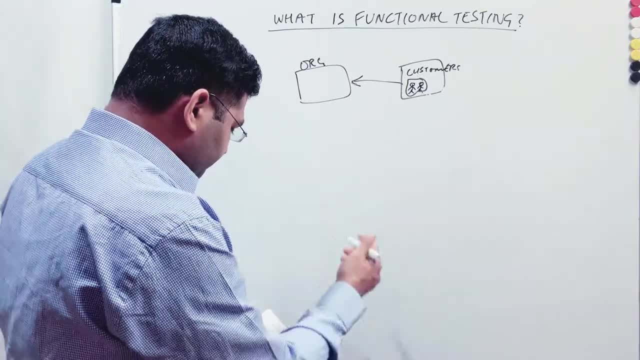 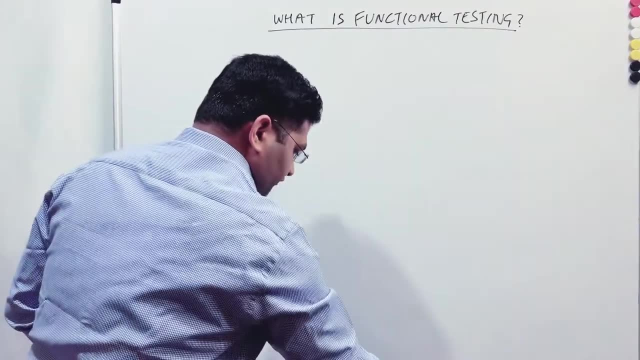 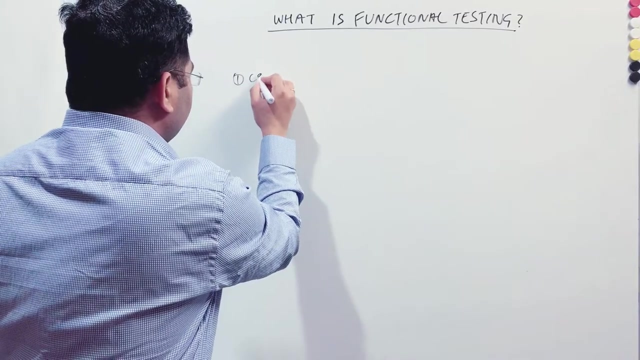 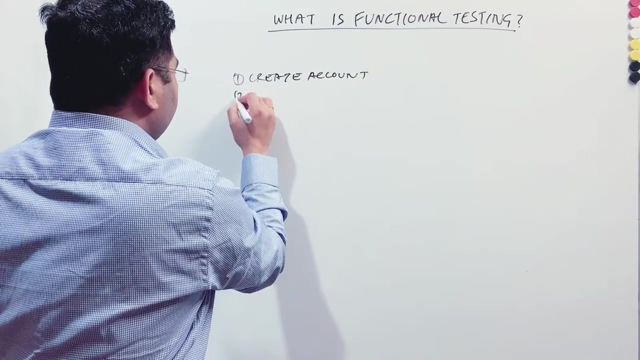 of the requirement is functional testing. So let's take an example here. So what I'll do is I'll take a couple of, you know, examples of Gmail. So usually if I talk about Gmail, so Gmail, let's say I have a functionality of create account, Okay, And then so create account functionality. 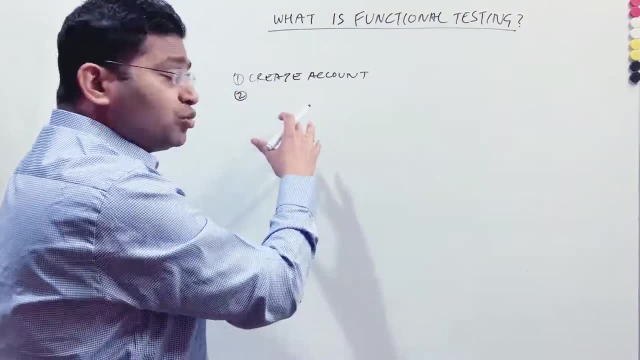 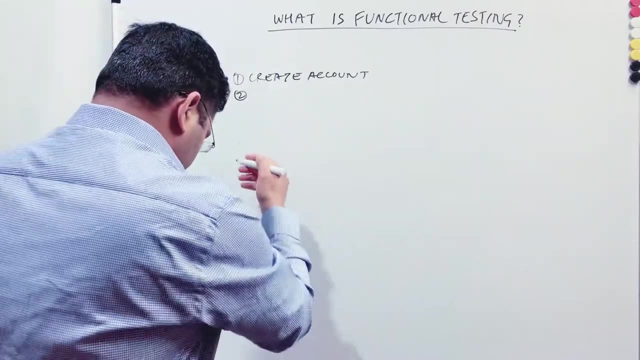 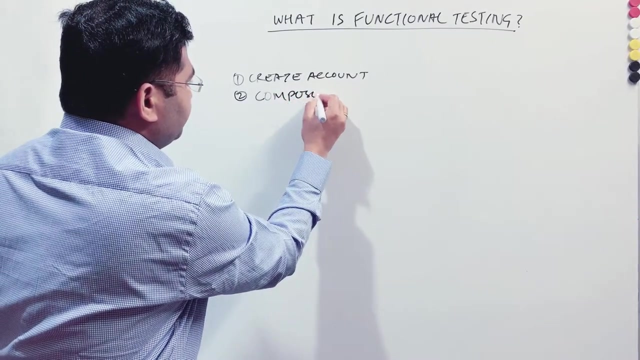 or feature will allow you to basically create the account for Gmail right So that you can draft email and send emails right. The next functionality could be: after you create the account, you should be able to compose email right So I can compose email. That is another functionality I can. 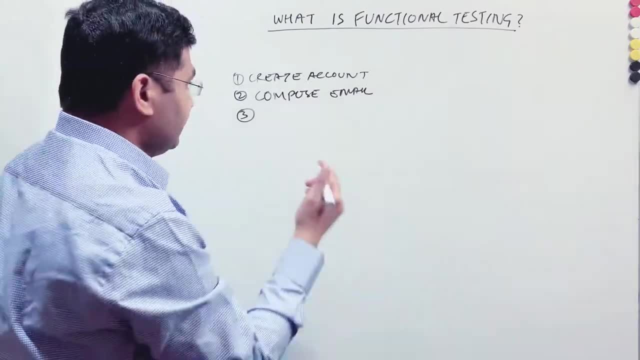 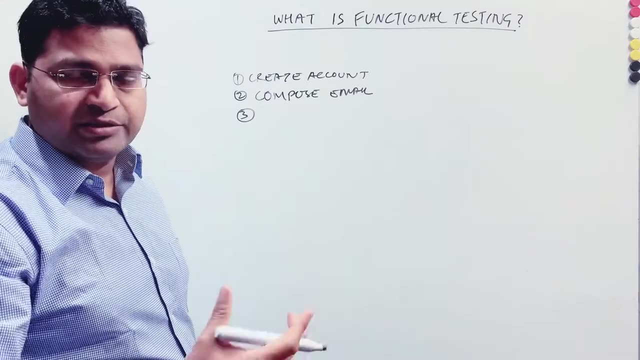 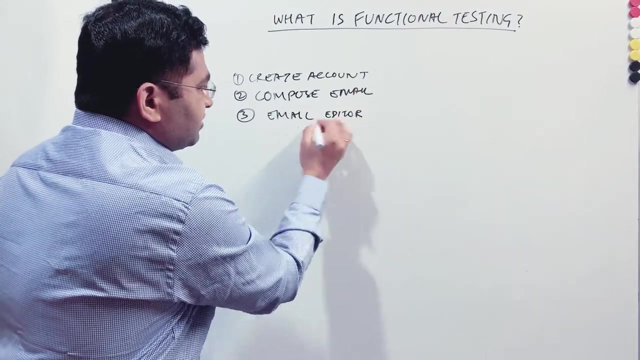 you know, have the functionalities or the requirements around the editor. So once I click on compose email, what all functionalities- editing functionalities- are available, I will in the email editor. right So? email editor, So that can have a lot many more requirements within it, right? So this is the high level. 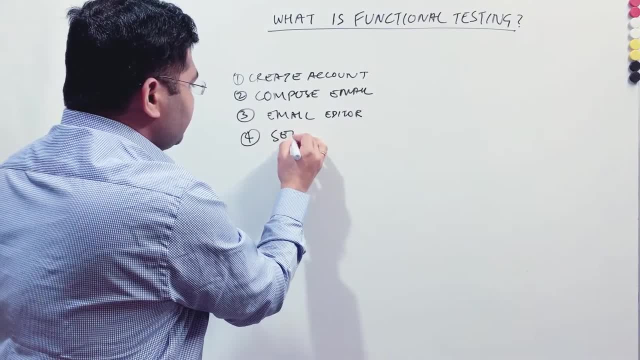 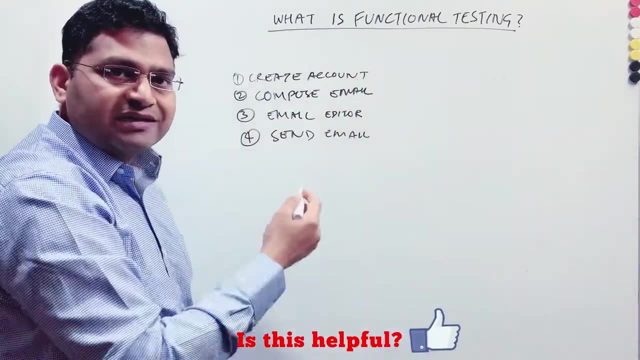 requirement that I'm covering. and then you know, send email, Right? So these are some of the you know functional requirement or the requirements that need to be verified in Gmail, Right? So if you are verifying this, create, 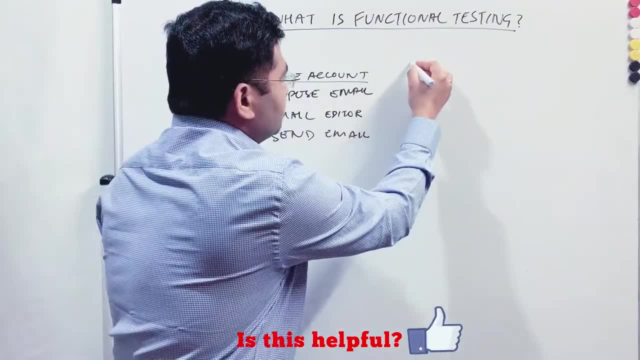 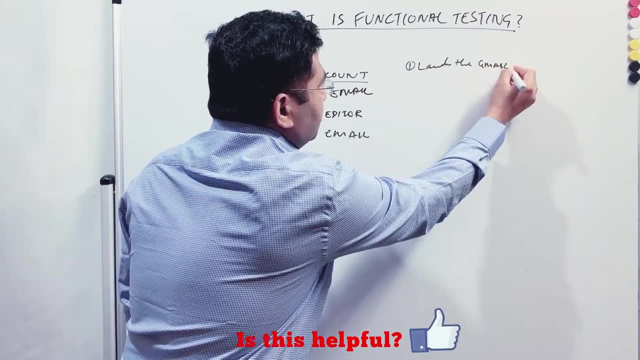 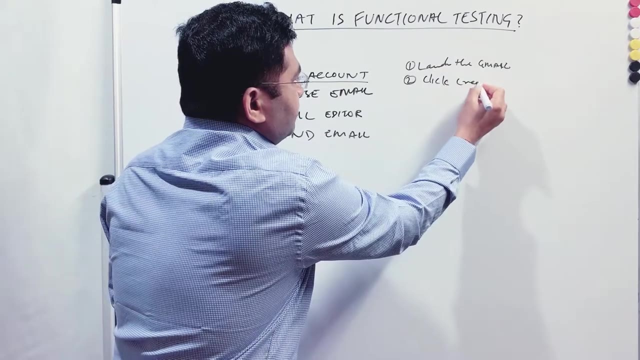 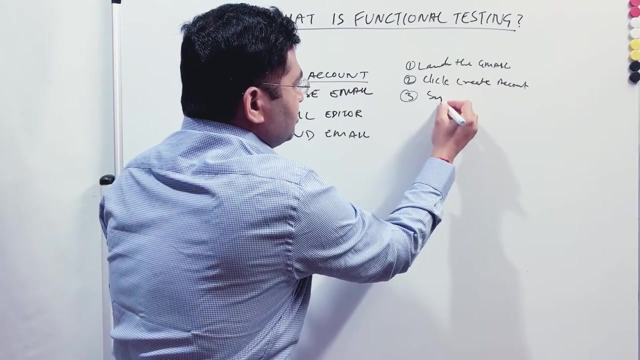 create account. so what you will do is you will follow certain steps and launch. so you launch the website, launch- you know Gmail, okay, and then you will click on create account. so click create account and then you will click on, you will supply all the details or supply user details, and in user details you 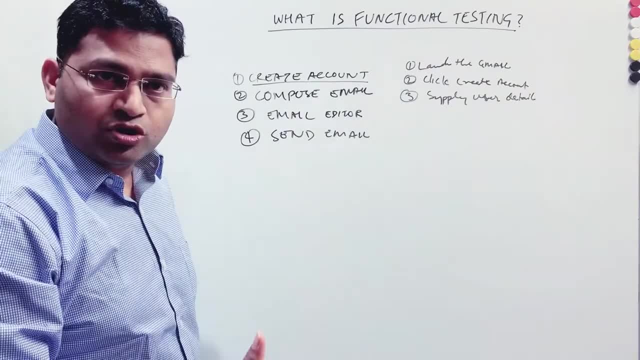 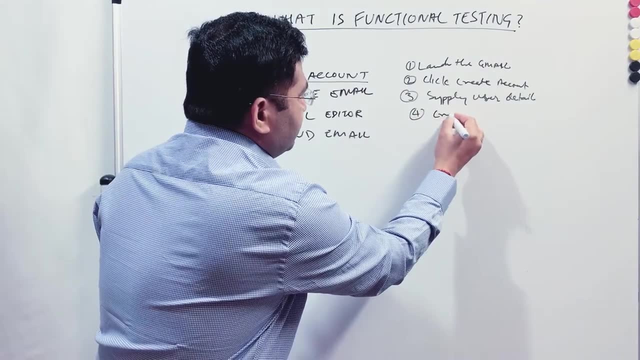 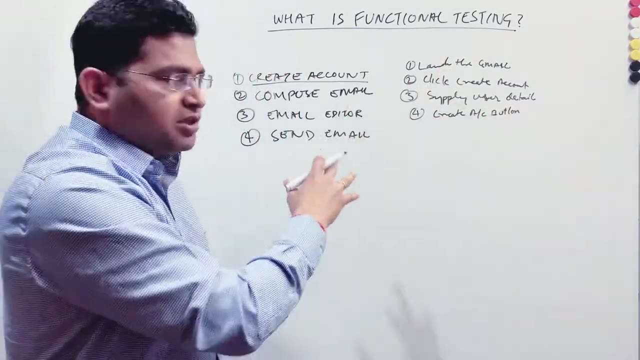 should even like first name, last name, what email you are looking for, the password, etc. so what all details are required? you supply all those user details and then you click on create account button, right. so these are the normal steps that you will follow to verify the account creation is being. 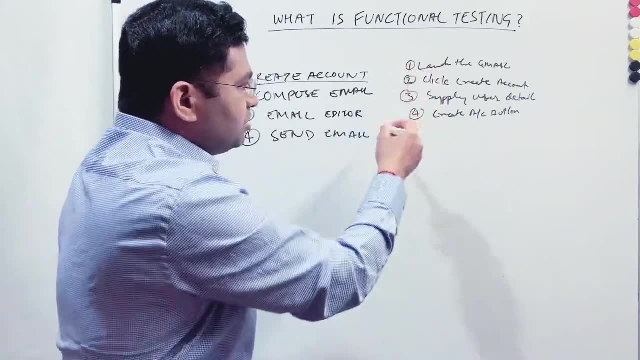 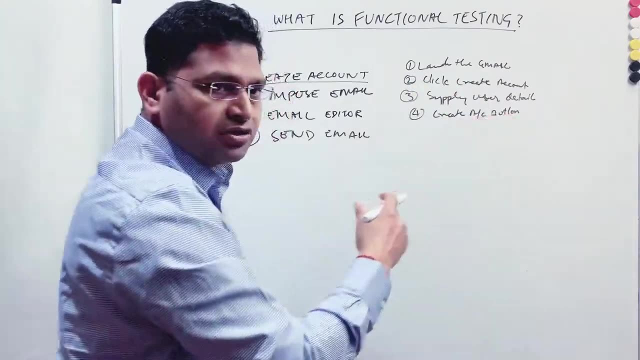 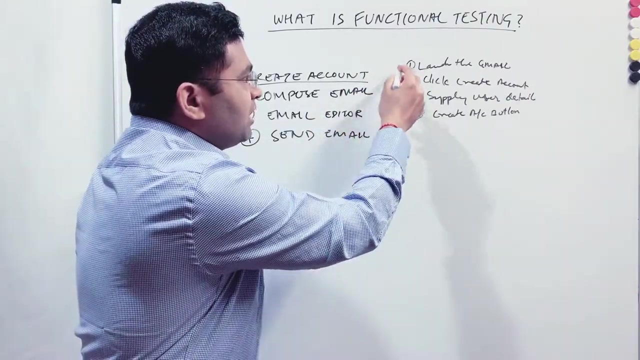 successful on gmailcom, right? so this is usually how the test case will look like. so you will follow certain steps, the process, and then you will verify that expected outcome. I try to cover how you will write test cases as well in future tutorials, but just to explain you functional testing. so we are following. 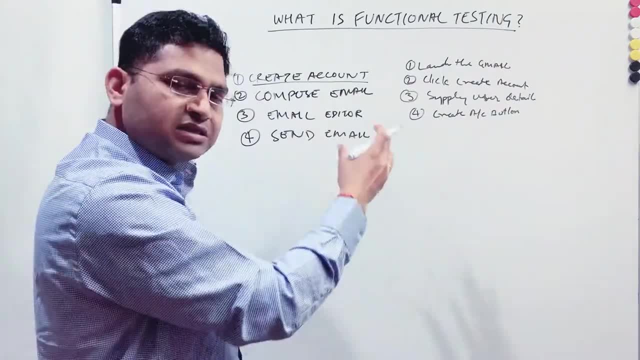 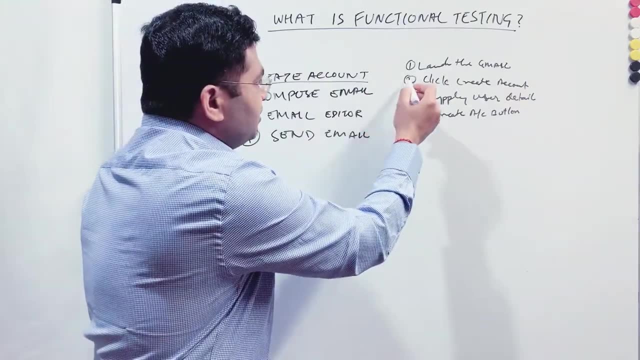 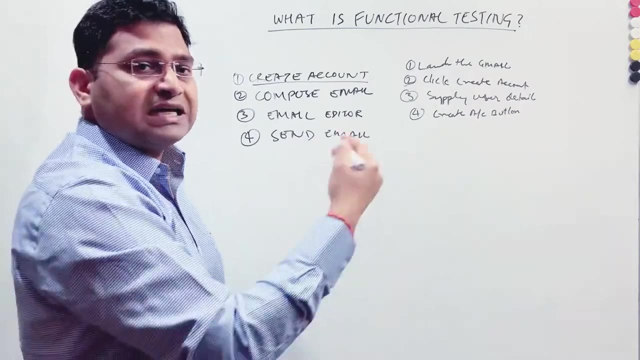 certain steps, which is basically nothing in the testing project. it's the test case and then, based on those test cases, we verify whether that test step has passed. now, each of these step is a test step, right? so whether these, if I launch Gmail, it should launch successfully. if it is, it has launched. that means that 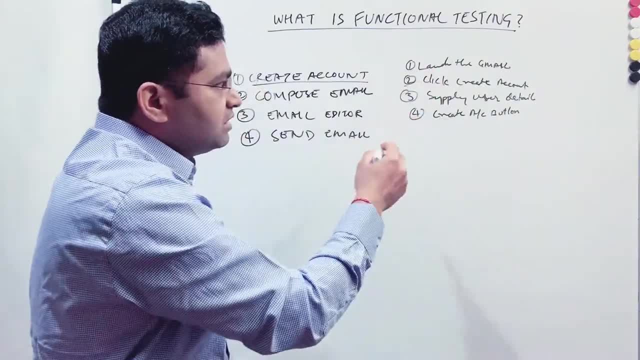 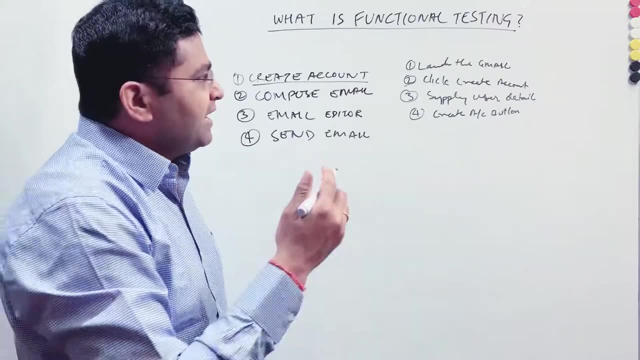 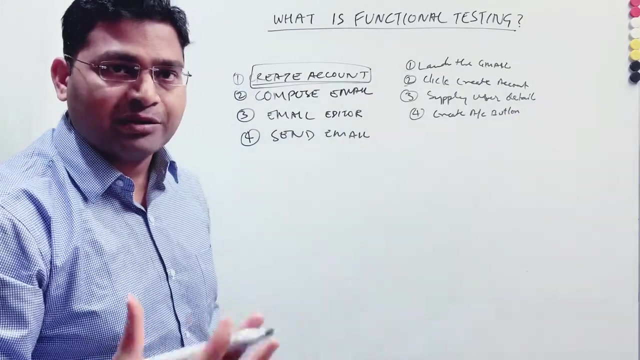 test step has passed. so when a tester is performing all these steps one by one and verifying that these steps are being passed, that is what functional testing is, and functional testing is verifying these requirements, or the requirements that need that are built within the application. right now, when we talk about functional testing, functional testing is: 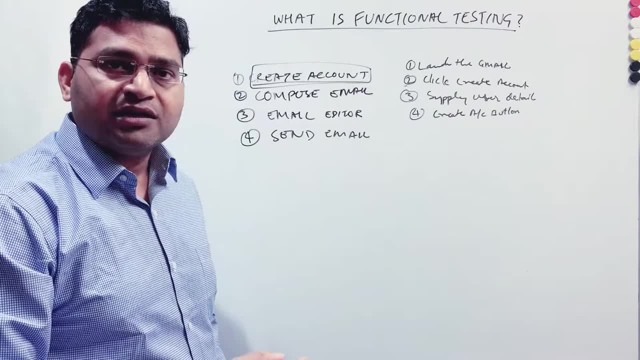 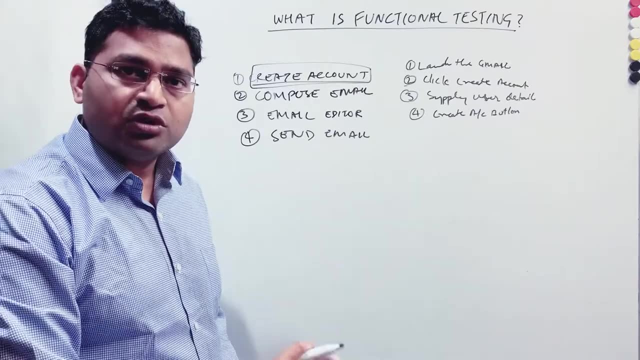 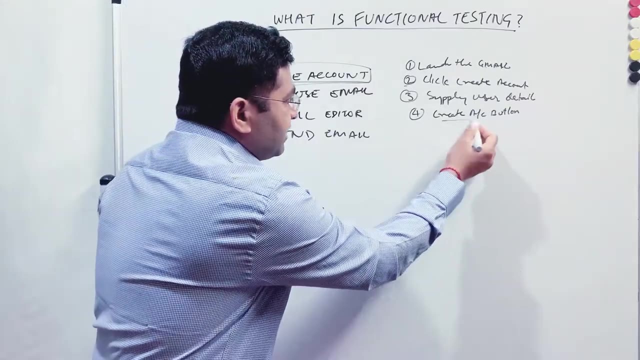 not, or the person doing functional testing is not worried about the non-functional aspect. for example, how is the performance? what is the response time? right? so you don't need to worry about the non-functional aspect of the account creation. so, for example, when I click on create account button, I am not worried about whether I am redirected. 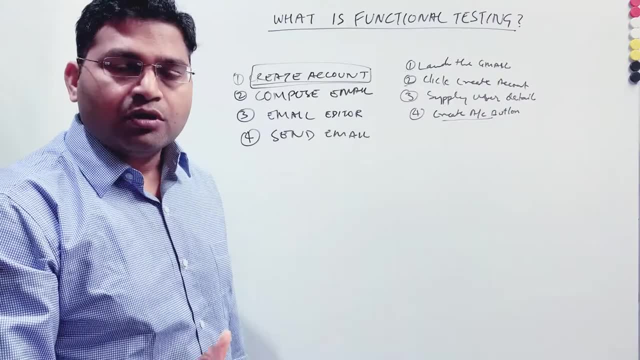 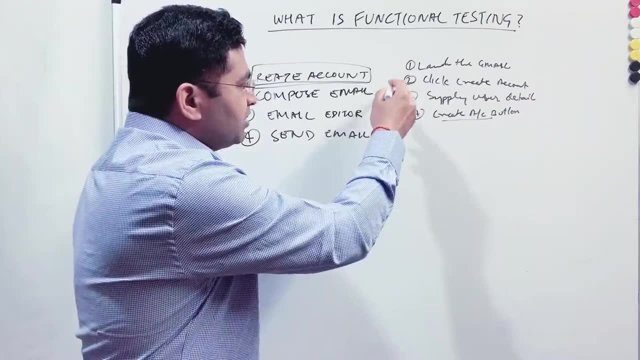 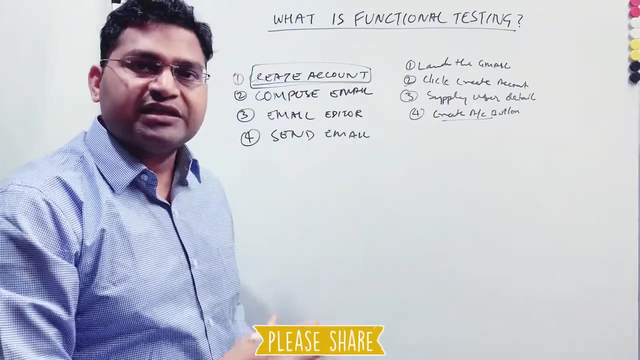 after 30 seconds to the actual account, or three seconds, right. so that needs to be tested as part of the non-functional testing. in the functional testing I am just worried about- or I need to cover that- the steps that I follow or the requirements that need that are being built in the application. 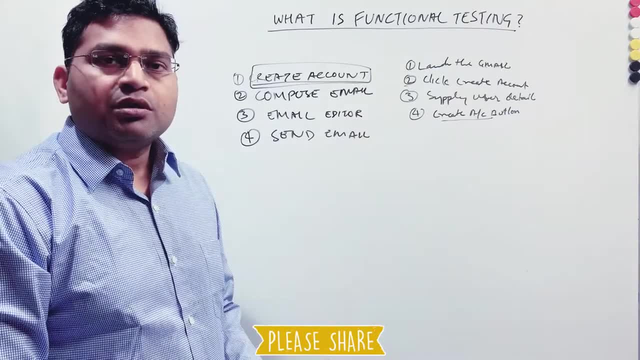 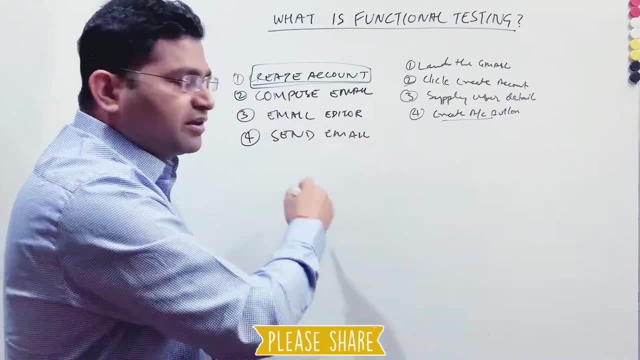 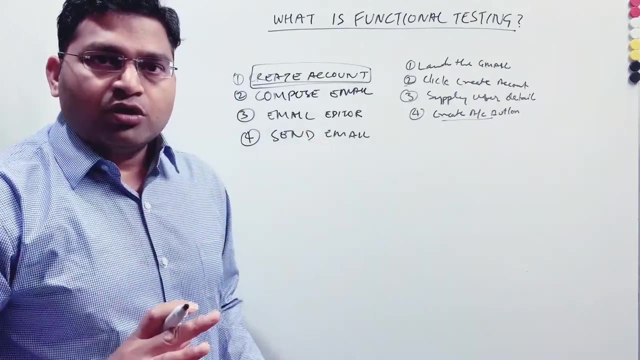 are being working properly or being fulfilled by the application developer or the development that has been done as part of the application. now, this is the live example that I have taken, but usually you can correlate with the actual scenario. so, for example, I am a new organization and I have a requirement to 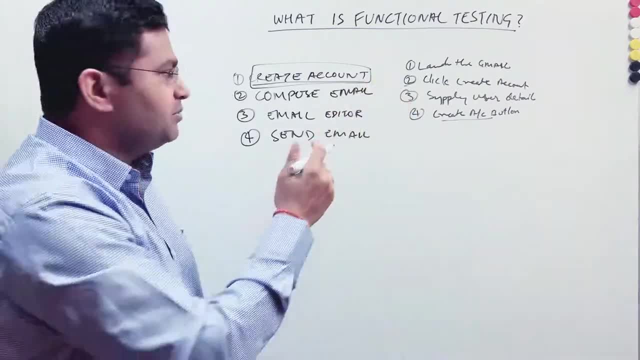 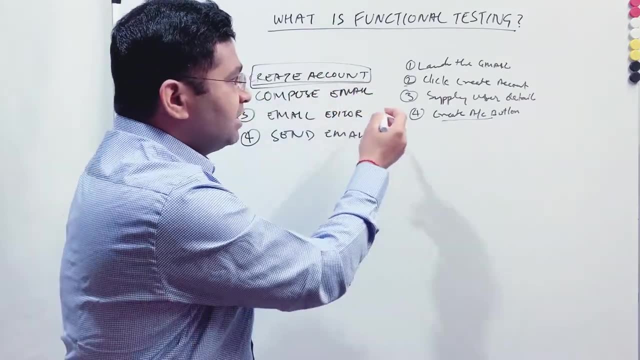 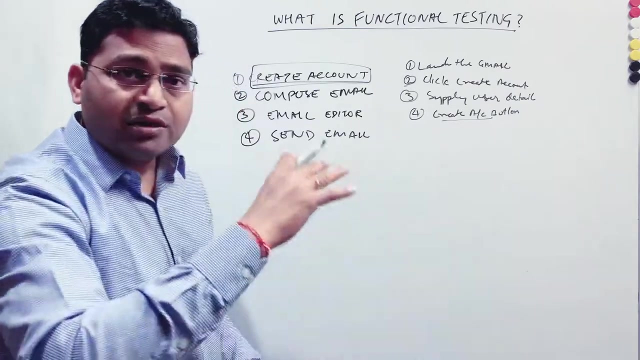 build something similar to Gmail. this is what I'll be getting as the requirement. so create account, compose email and in the requirements document, all the details will be provided right. so, for example, when create account button, what will be the text on it, and then in the supply user detail, how the form will look like. what all? 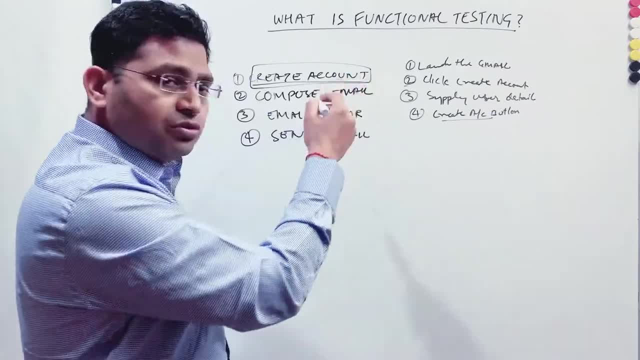 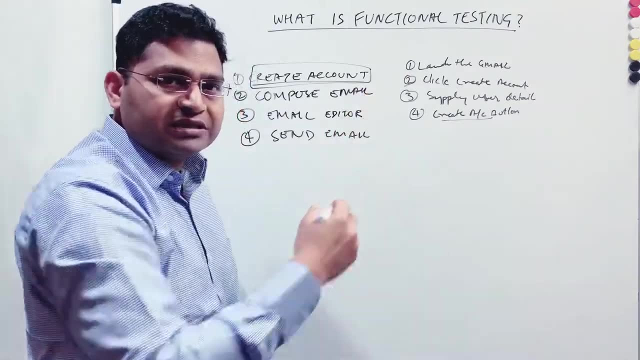 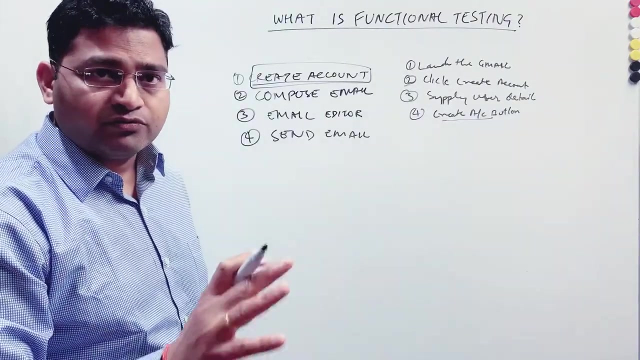 fields will be there. so all these details will be provided in those requirement and when, as a testing team or a test team member, I'll verify all those when I run those test cases. okay, so this is what functional testing is, and functional testing is a very important aspect of software testing. 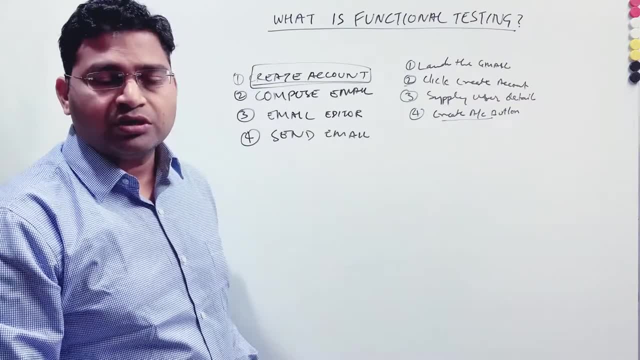 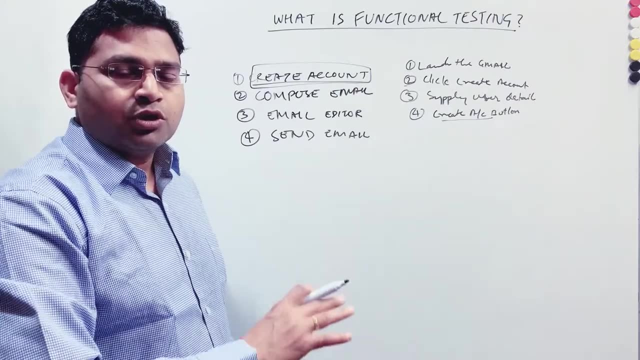 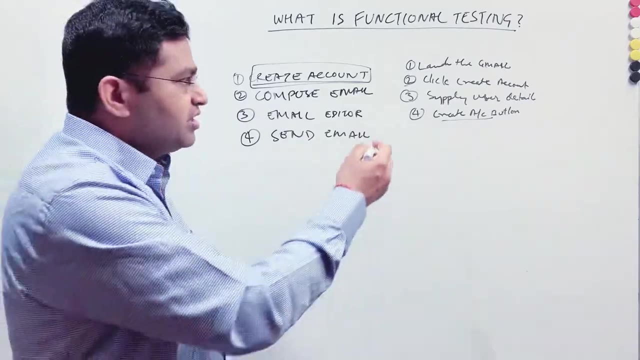 because most of the time when you start your career into the software testing you'll be doing, you know, functional testing first before you can actually- you know, you know- go ahead and automate the functional testing right. so it's basically a manual testing, manual verification of the features and functional testing is black box testing. 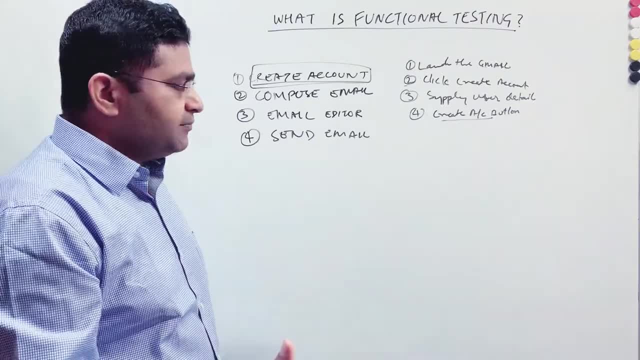 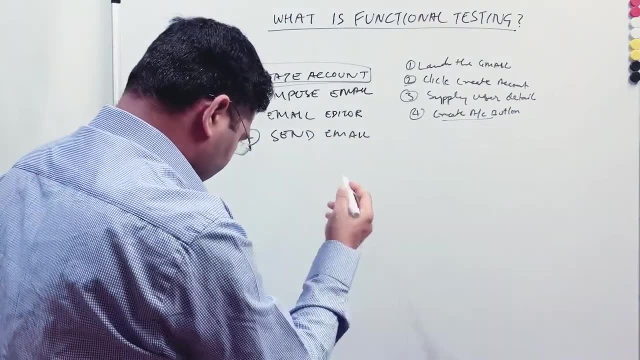 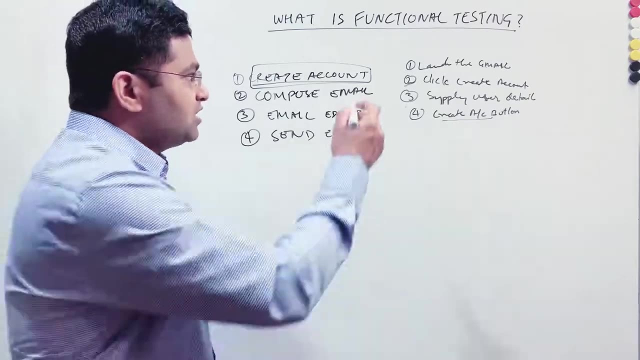 so I'll cover what exactly black box testing it is in upcoming tutorial as well. right, so this is a brief about you know what the functional testing is, and and other important thing about function testing is that it can be automated easily. so once say, for example, you follow all these steps here. right, so this is all ui. you know that gmail can. 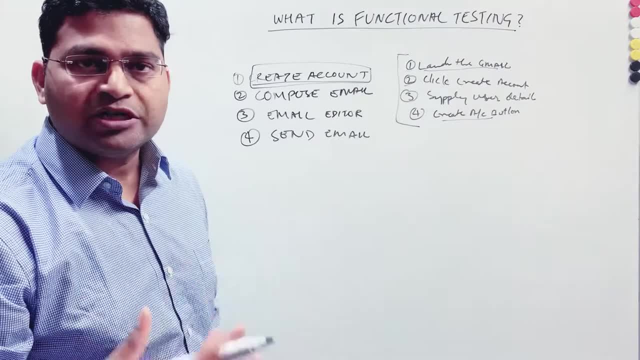 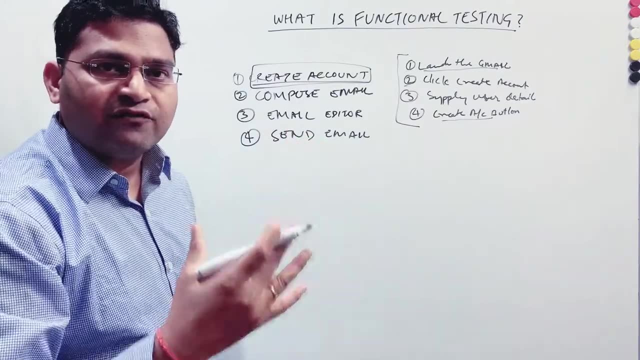 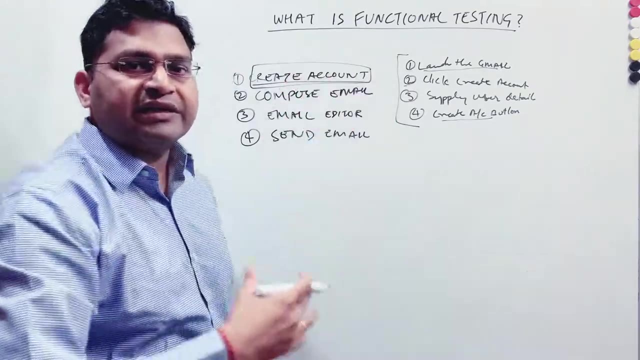 be open in any browser. so this is ui. there are a lot of tools to automate uis. selenium is very popular, so you can. once you verify that all these functionalities are working fine, then you can use any automation tool and go ahead and automate these steps so that next time you can easily.